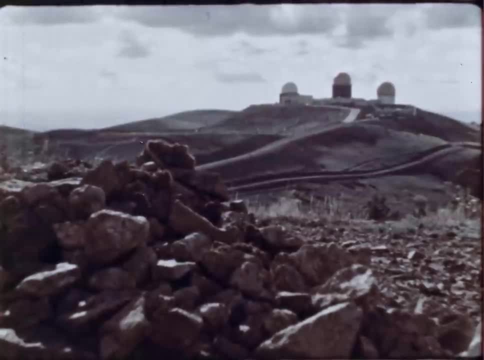 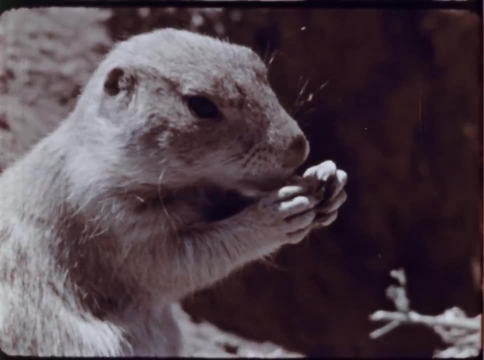 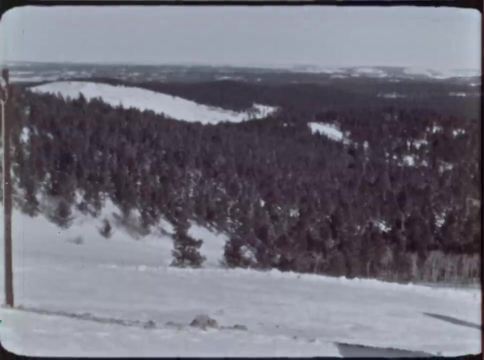 facilities. The installation is in remote country Sundance Wyoming. the nearest settlement is six miles away, At Warren Peak. neighbors are few. PM-1 was placed here to prove that it could function in isolation in a climate nearly. as rigorous as that at the poles. At 6,000 feet above the sea, the temperature ranges from highs of 87 degrees Fahrenheit to lows of minus 50. But the radars must read the skies in any weather, And PM-1 will furnish them power. 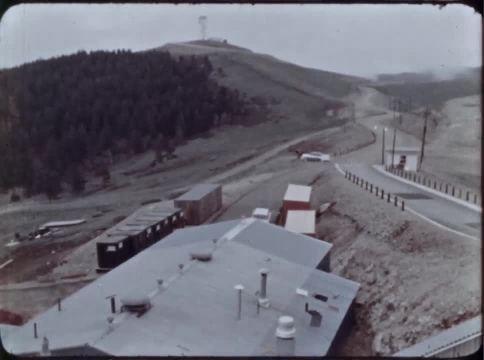 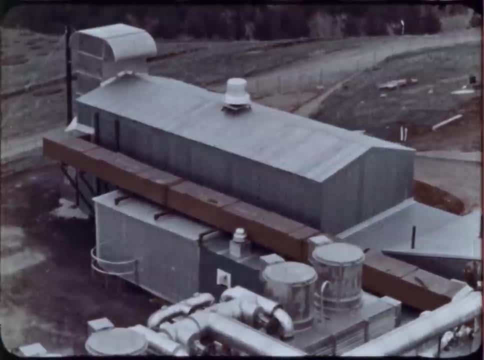 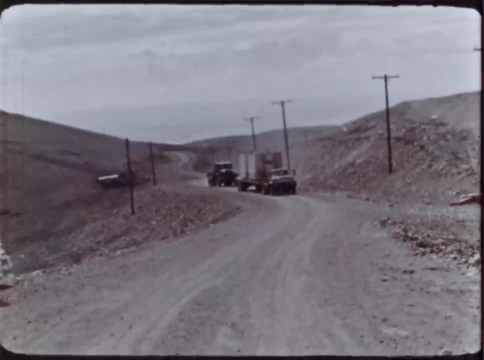 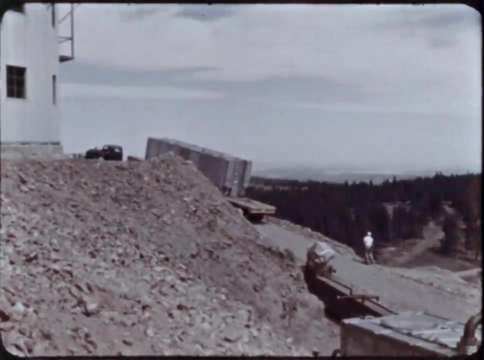 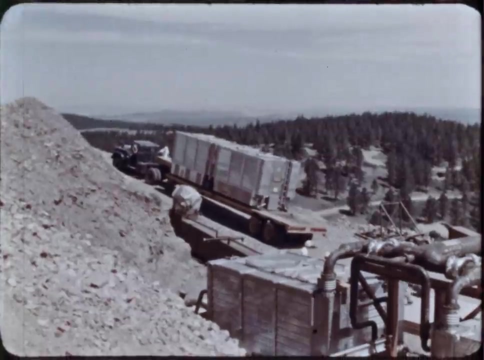 For two years from a single nuclear fuel loading. This reduces the need for heavy logistic support. Supplies reach the base by road, 93 miles over land from the rail head at Rapid City. The basic plant was assembled at the site from 16 packages. It could be relocated. the same way, And so 4 packages miscellaneous equipment. but the heart of the PM-1 is in the remaining 12 packages, divided into the primary and secondary systems. The primary system is made up of three of these packages. There are four tanks, reactor, steam generator and spent. 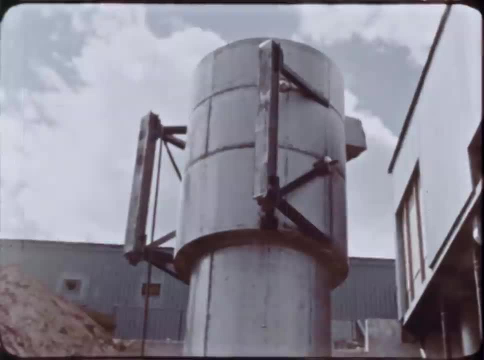 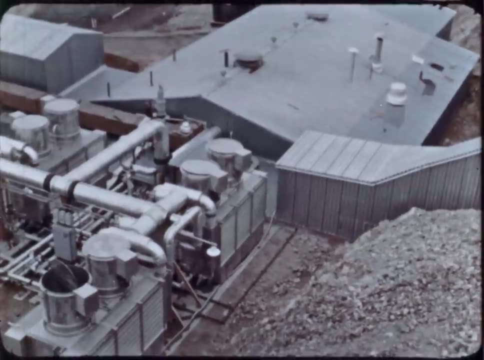 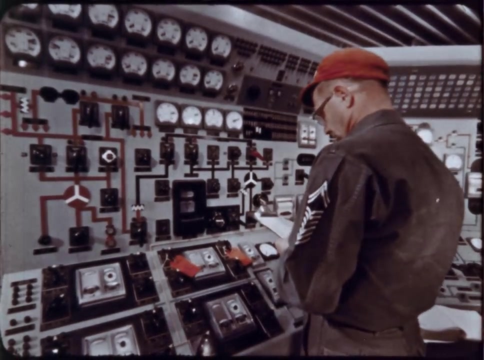 fuel core tanks grouped together. The radioactive waste disposal tank is a part of the third package. It is shipped in the spent fuel tank. The secondary system contains nine packages. The control room package contains the console from which the plant is run by a single controls operator. These controls 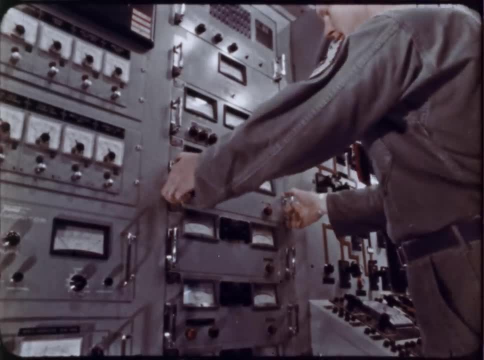 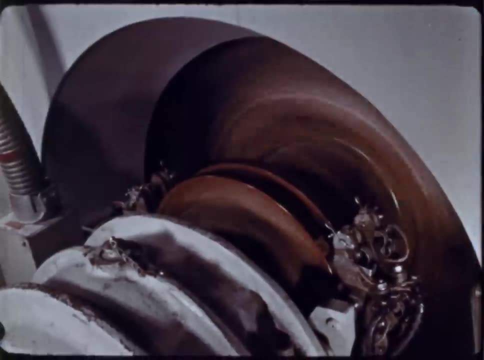 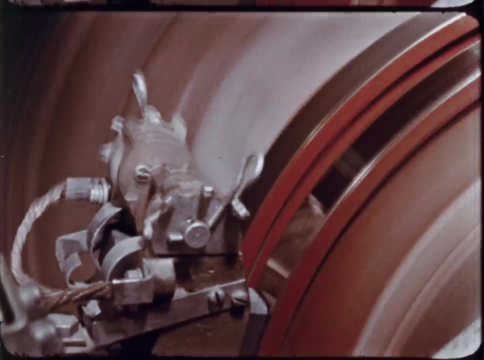 must meet a reliability specification of 99.45%. Consequently, solid-state components are employed. The turbine generator package houses the equipment that converts to electrical energy the heat and the heat generated by the reactor core. The generator produces 1250 kilowatts gross. 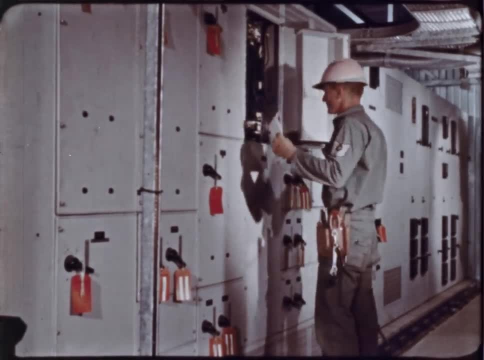 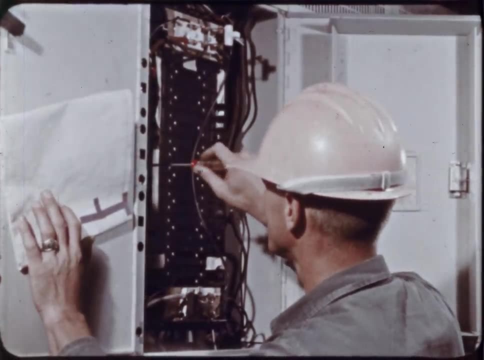 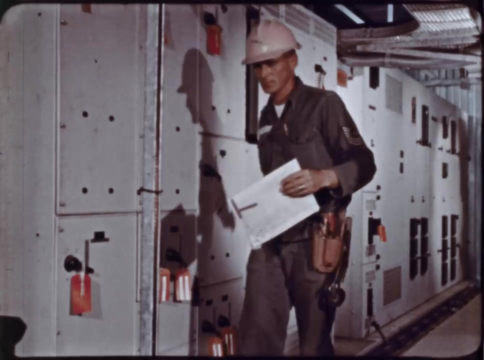 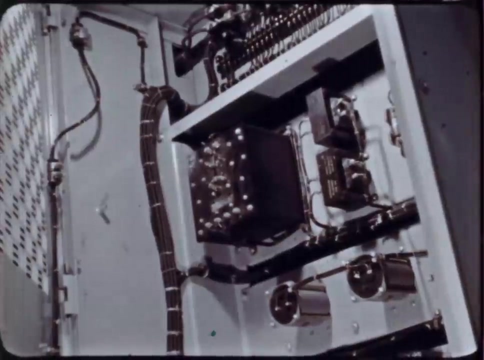 output. Equipment in the switch gear package works with the generator to refine this output and to give the plant one of its most striking design characteristics: the high quality of the electricity produced. This quality is governed by a voltage regulation and a static exciter. The voltage is determined by a voltage regulator and 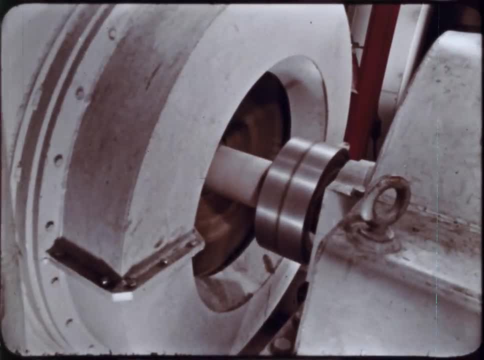 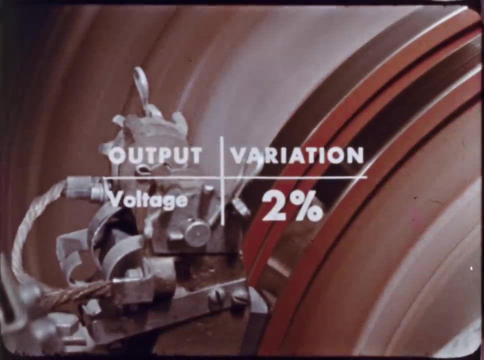 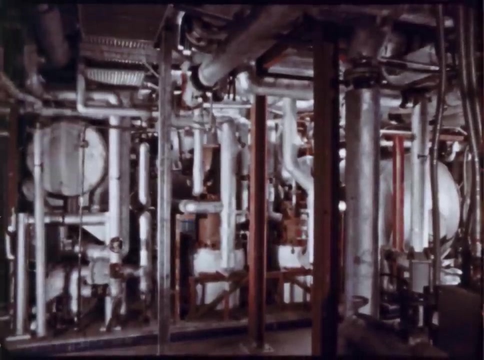 static exciter which can eliminate the need for further electrical refinement. With these units, electrical variations are held to tight tolerances. Voltage varies less than two percent. frequency less than two percent harmonics less than two percent units. One contains the evaporator reboiler which manufactures the low. 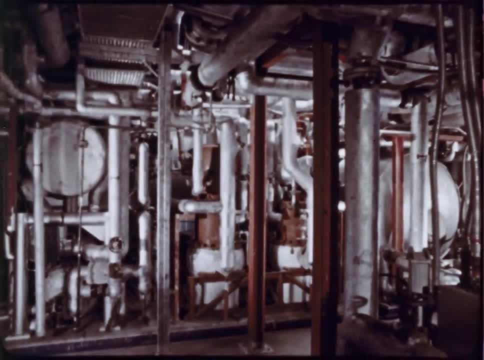 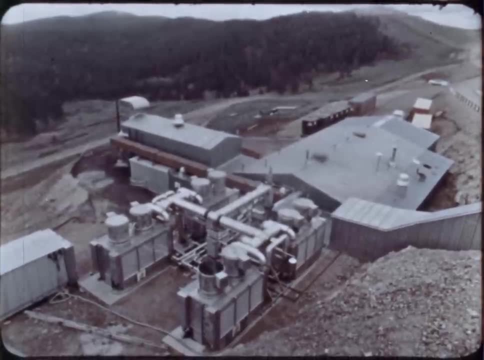 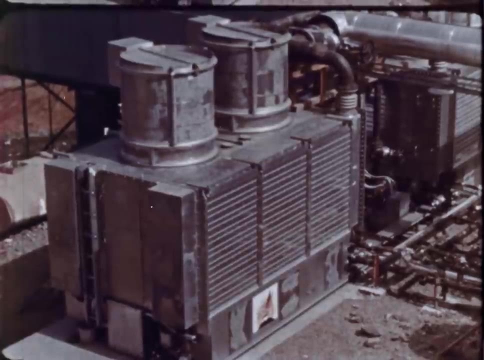 pressure steam for space heat. The other unit is conventional heat exchanger equipment. Four direct air to steam condensers account for two packages of the system. They cool the steam from the turbine by drawing air over the condenser piping. No cooling liquid is involved. This type of condenser was 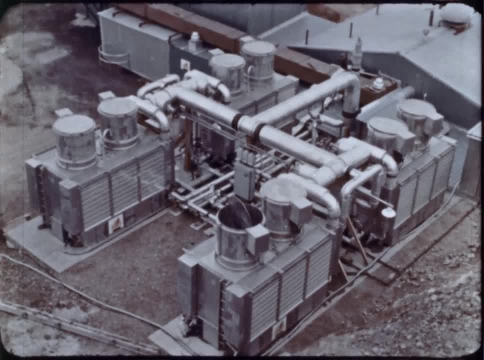 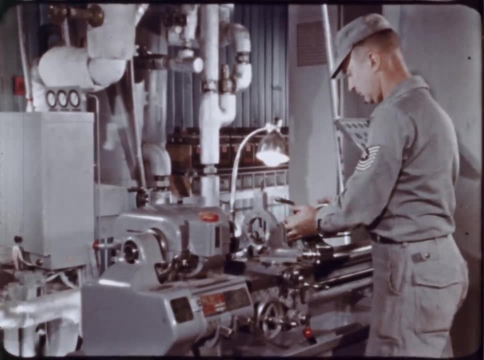 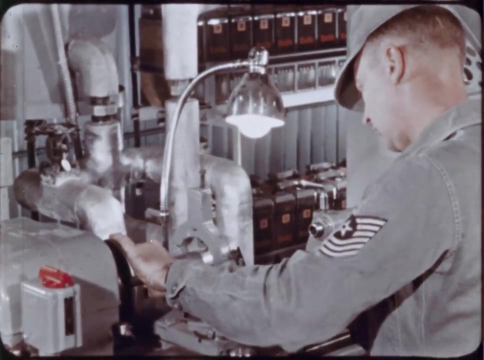 selected so that the plant can operate in an area with a low water supply. The maintenance package holds standby generating equipment and a shop with a grinder, welder and lathe. Almost any general repair to the plant can be made here By specification. the plant can only be shut down 21 days per year and of 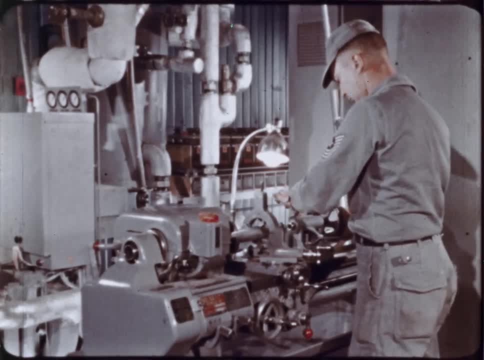 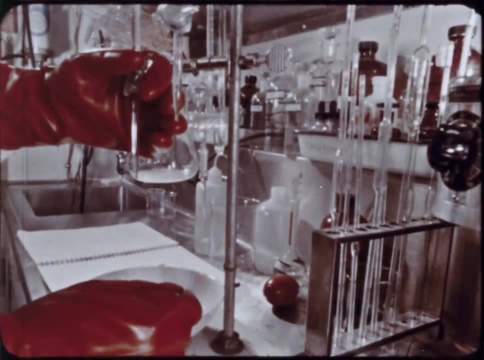 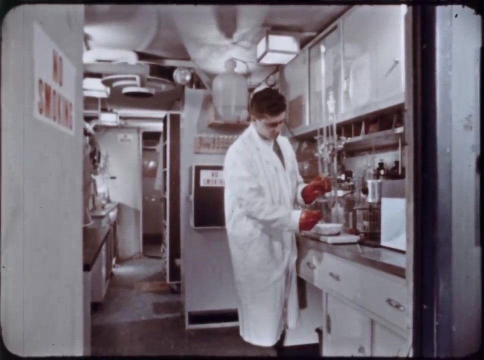 these only six are scheduled for annual plant shutdown. The shop will help the plant to meet its shutdown specification. A separate building holds the ninth package of the secondary system, The decontamination and water chemistry unit. Here too, health physics sets its line of. 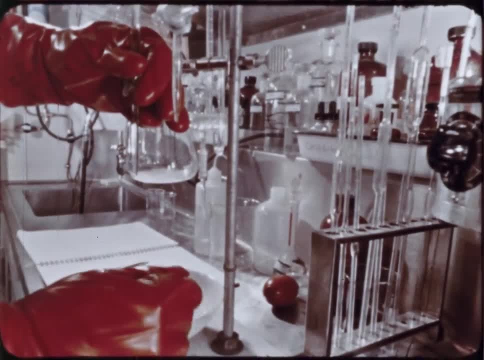 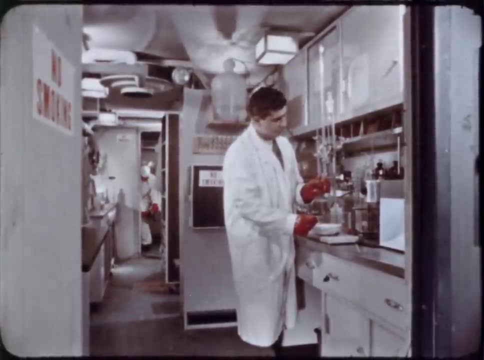 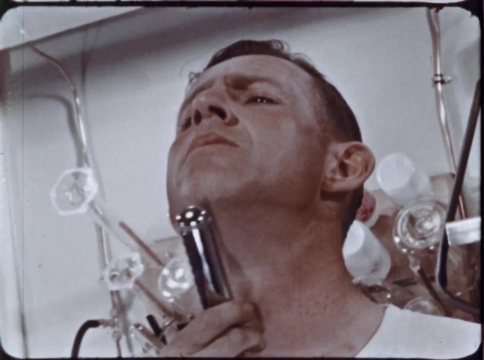 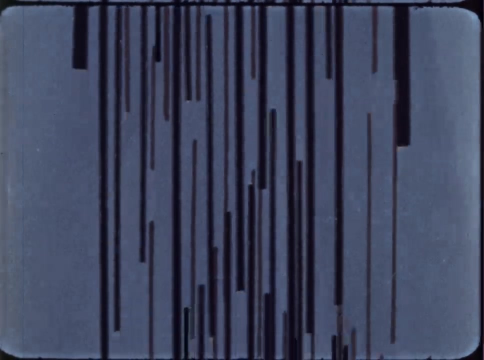 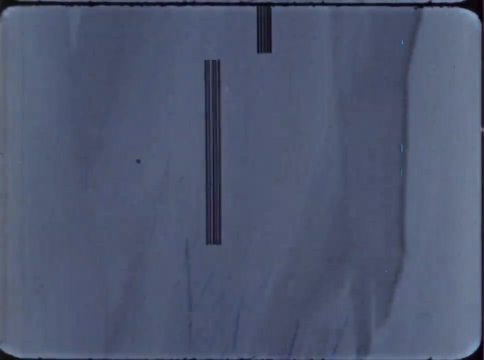 demarcation establishing the contaminated and clean areas. Personnel crossing this line from the primary system are given a radiation count. We are now ready to look at the design of the system in some detail. 741 nuclear fuel tubes make up the reactor core. These tubes are grouped into seven fuel. 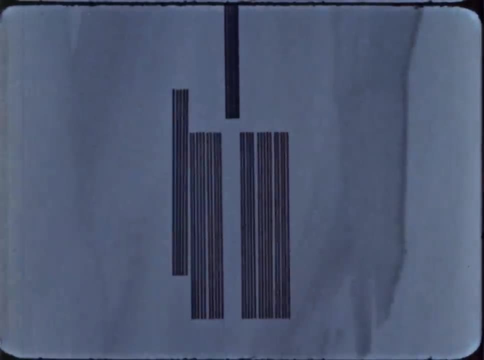 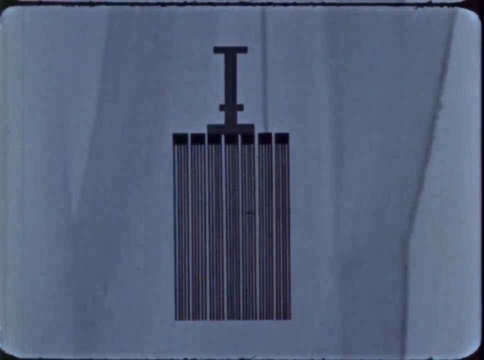 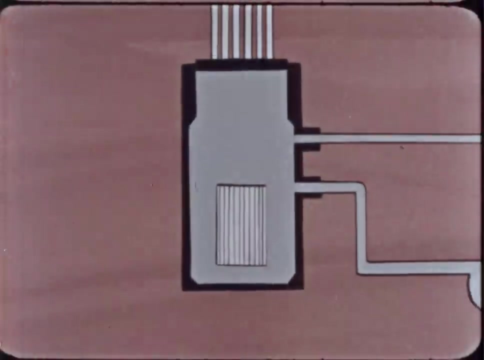 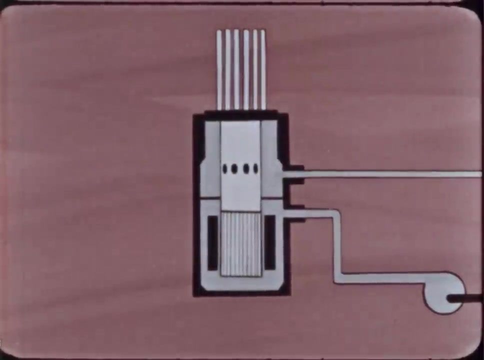 bundles- six peripheral and a center bundle- With the proper tools, we can fuel and refuel the core as a whole or, if necessary, we can replace individual bundles without removing the entire core. The core, a thermal shield and an upper skirt are enclosed in a pressure vessel. 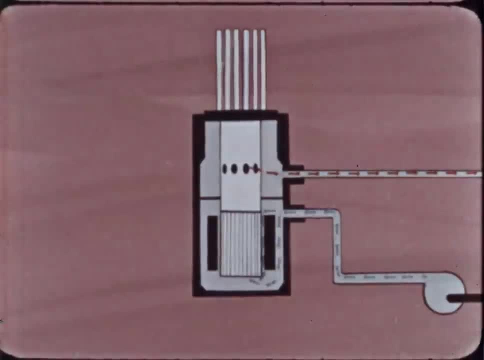 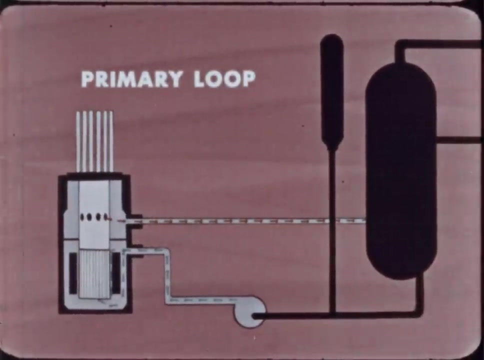 Primary water flows into the pressure vessel down around the core, cooling the thermal shield. This water then passes up through the core, absorbing heat and flows out the holes of the upper skirt. The primary water is conveyed to the tube side of the vertical shield. 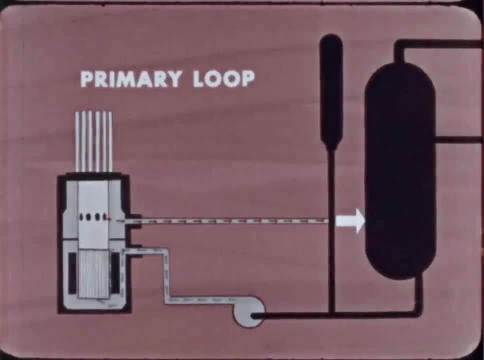 steam generator. It is pumped back by the primary coolant pump at a rate of 2,125 gallons per minute. Water leaves the reactor at 479 degrees Fahrenheit. It returns to the core at 447 degrees. A 32 degree rise in temperature means that the reactor generates nearly 35 million BTUs A pressurizer. 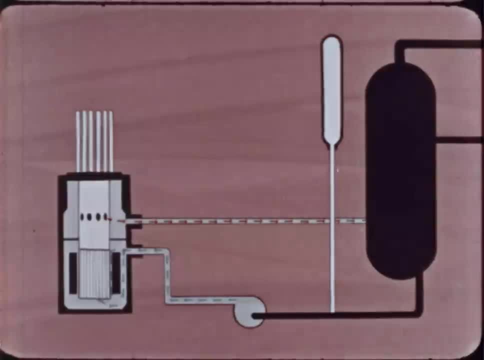 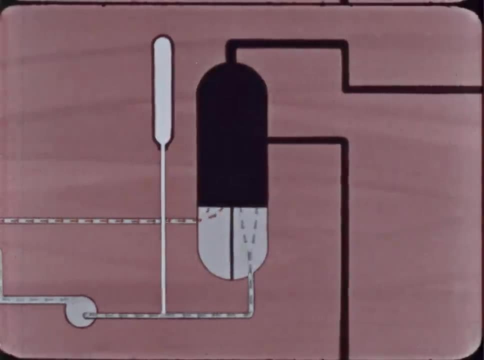 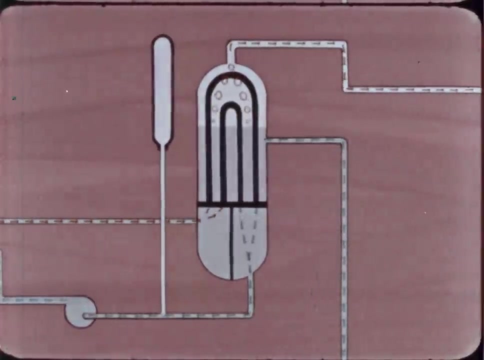 maintains the system at 1,300 PSI to prevent boiling. As the primary water flows into the tube side of the steam generator, it gives up heat and flows out. Secondary feed water picks up that heat on the shell side and is released as dry steam. This steam drives a 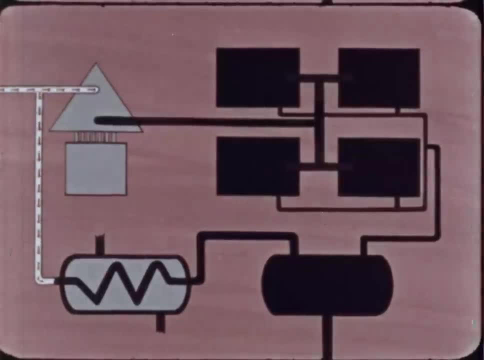 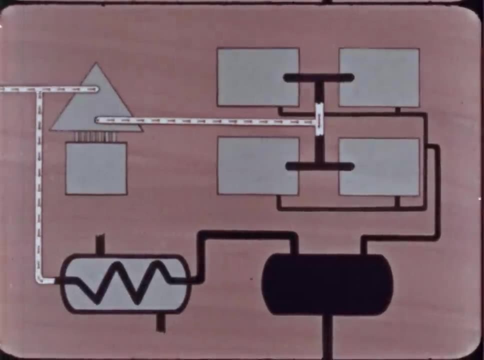 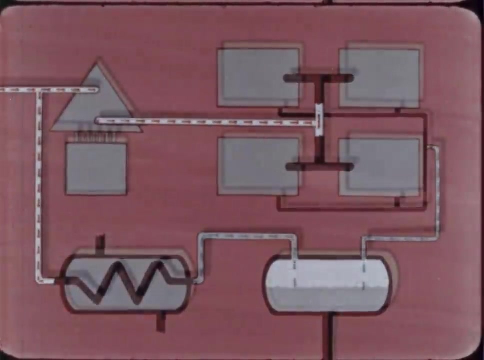 single extraction turbine generator and feeds the evaporator reboiler. at the same time, Exhaust steam from the turbine. Exhaust steam from the turbine flows to four air-to-steam condensers and is converted to water, which is drained to the hot well along with the evaporator condensate. 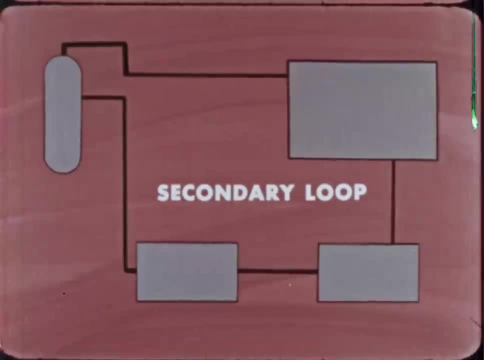 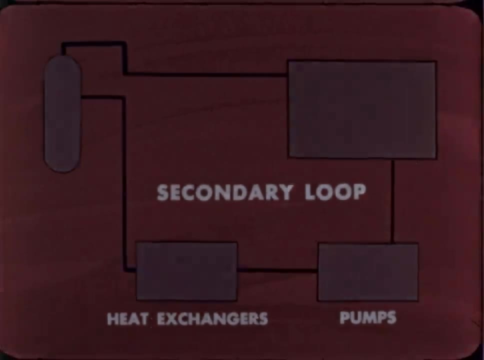 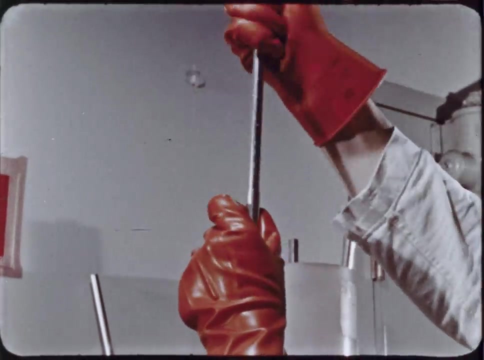 The remainder of the secondary loop is somewhat conventional, having the necessary pumps and heat exchangers to recycle feed water back to the steam generator. The fuel elements are basic components of PM1. Their manufacture starts our survey of PM1 fabrication and testing. 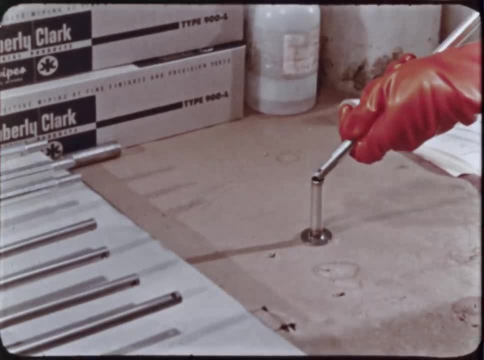 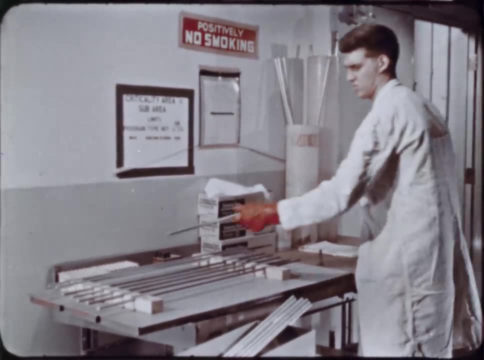 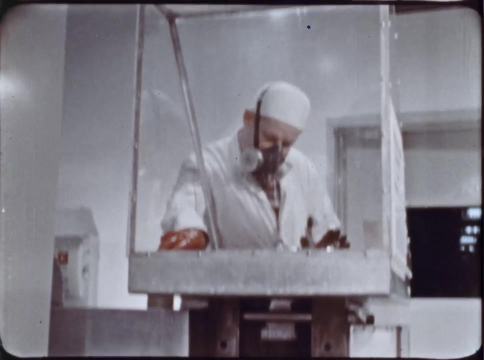 The fuel element tubes are approximately one-half inch in outside diameter and 33 inches long, of which 30 inches is a fissionable U-235.. We begin with the uranium powder. Each fuel element tube contains 40 grams of enriched uranium-235.. 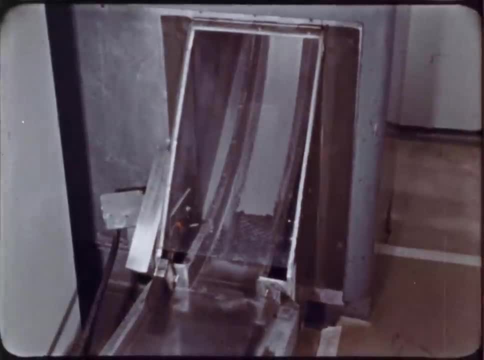 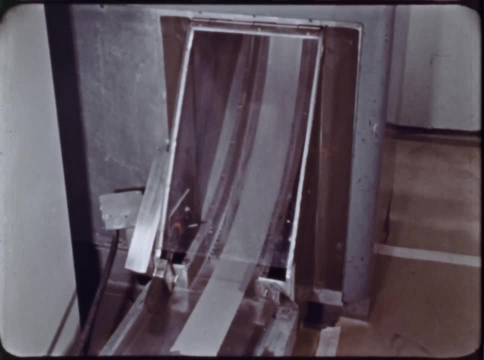 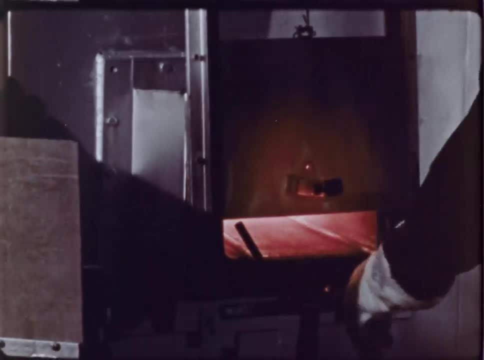 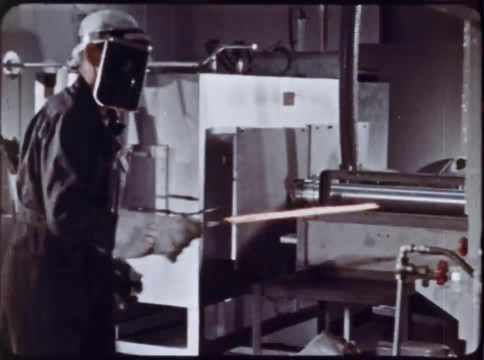 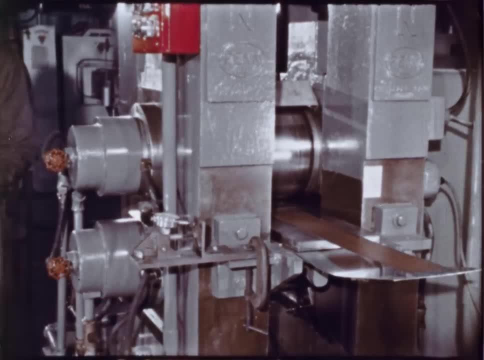 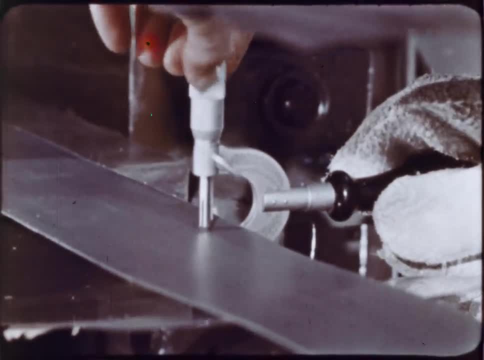 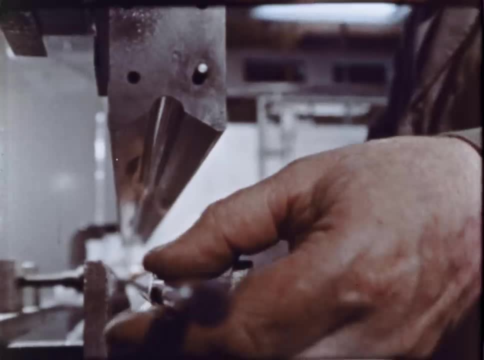 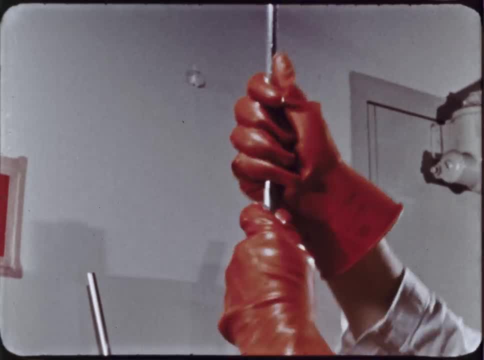 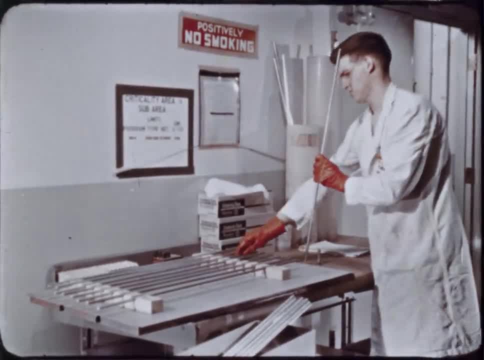 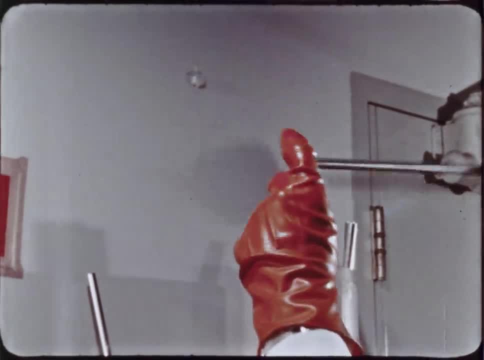 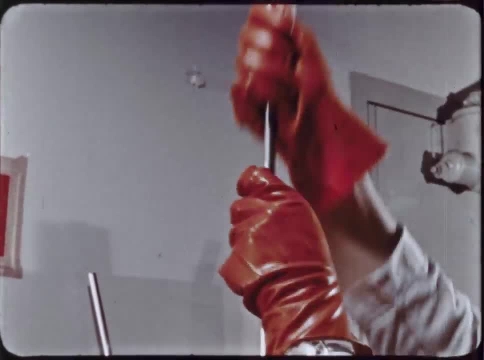 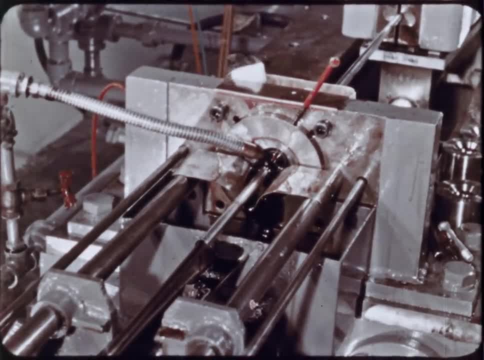 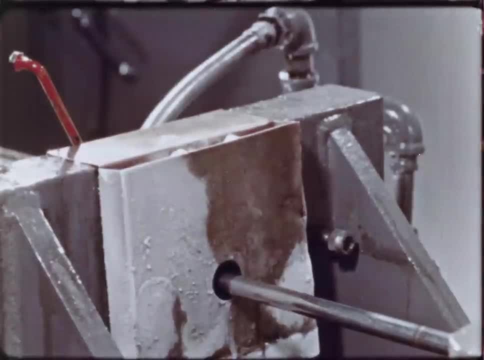 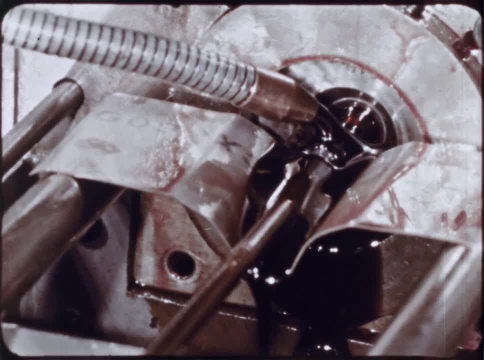 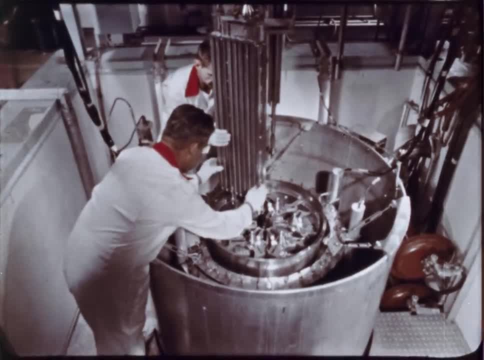 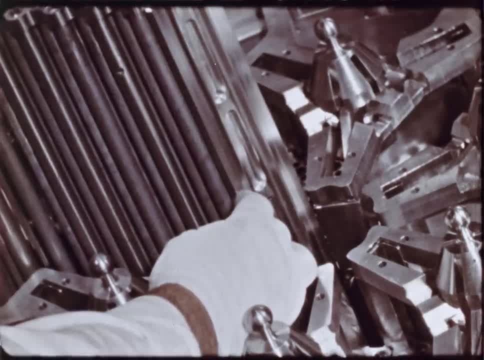 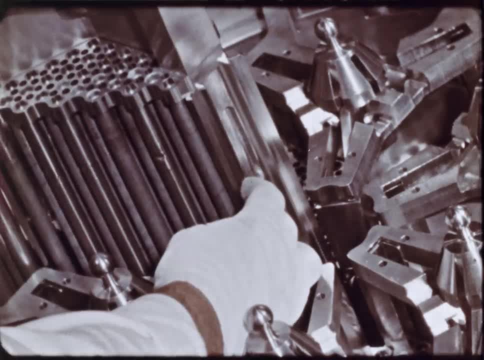 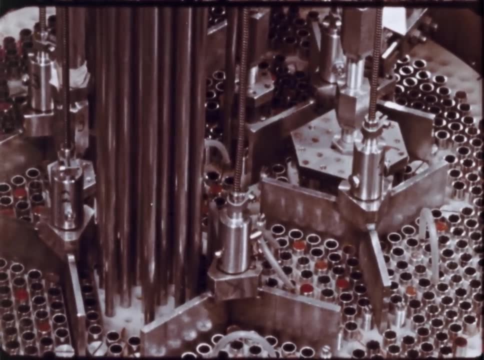 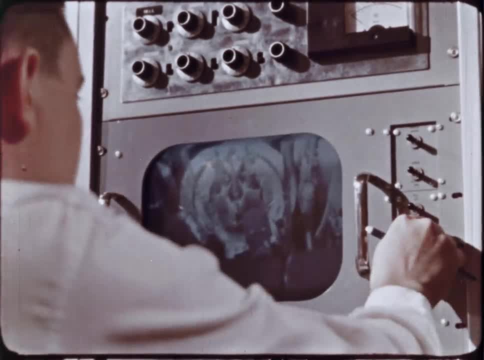 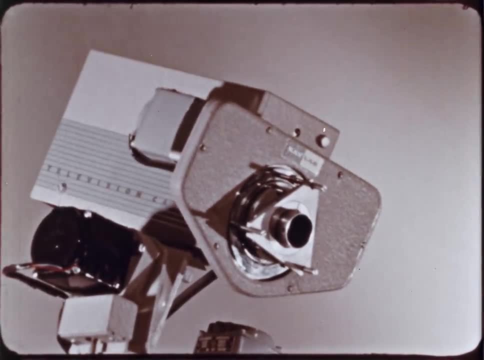 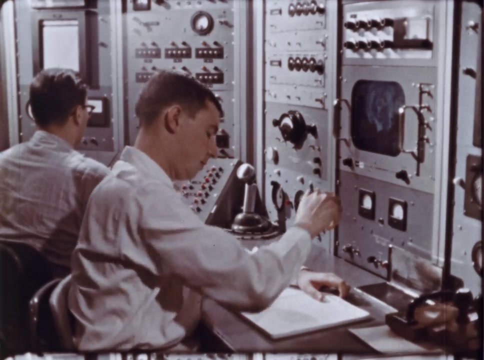 The chain reaction has begun. A test configuration of the PM-1 core achieved criticality for the first time on March 17, 1960.. These criticality tests gave engineers the basis for refining their design core configuration and checked out the effectiveness of the components that 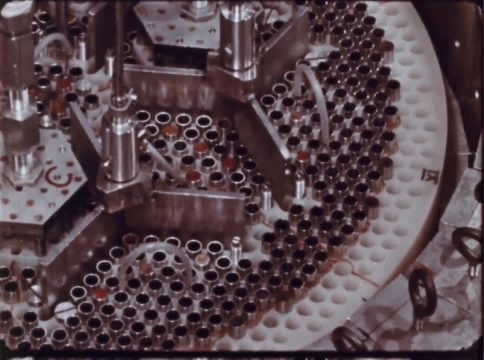 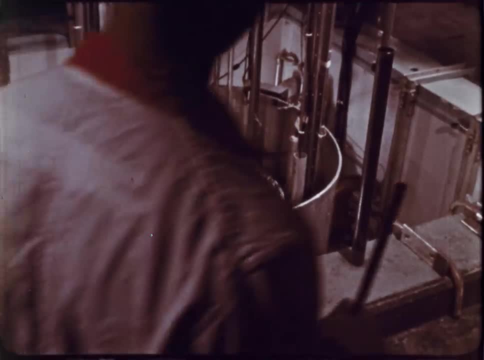 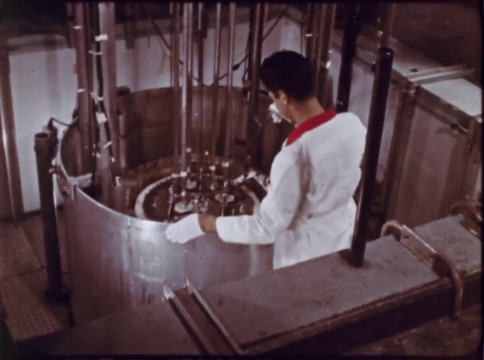 control reactivity in the core. The final configuration contains 741 fuel elements. Its diameter just under two feet. Its active length 30 inches. Its overall length 33 inches. 90 boron poison elements are permanently installed in the core. These burnable elements absorb surplus neutrons released by the fission. 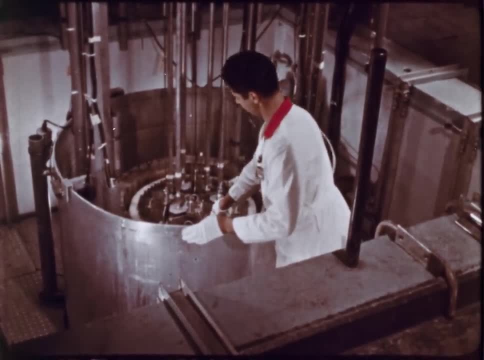 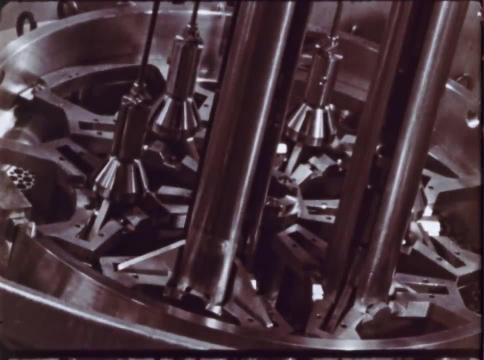 process. They decrease the reactivity of the operating core to a controllable level. Y-shaped control rods start, stop and control the rate of reactivity. The Y rods contain europium oxide stabilized with titanium oxide and mixed with stainless steel powder to form a cermet. There are six of these rods in the core. 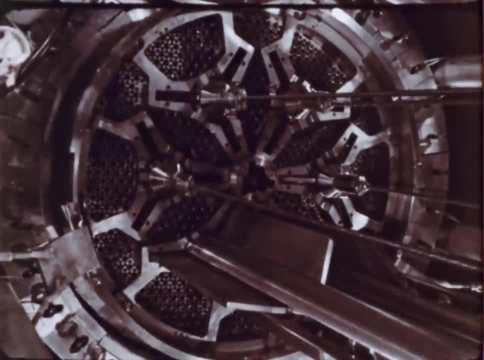 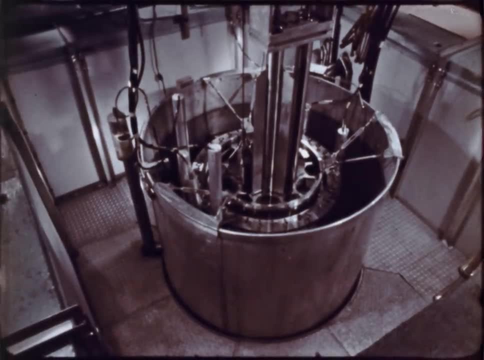 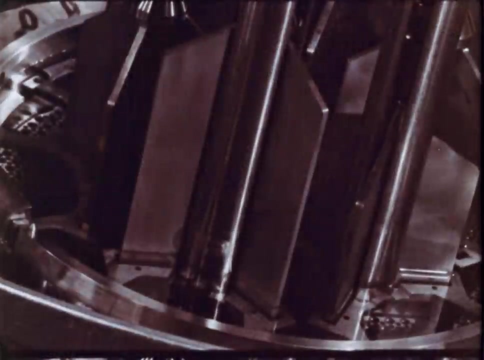 A reactor is subcritical. Fission cannot take place As a safety margin. the core is subcritical with only five rods fully inserted, or even with four rods inserted and two in the operating position. When all six are withdrawn, a point is reached. 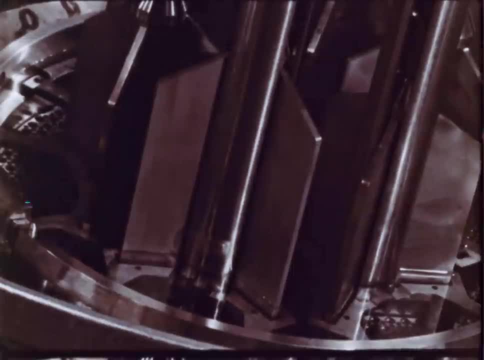 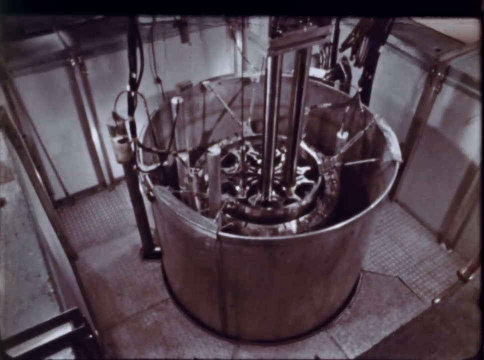 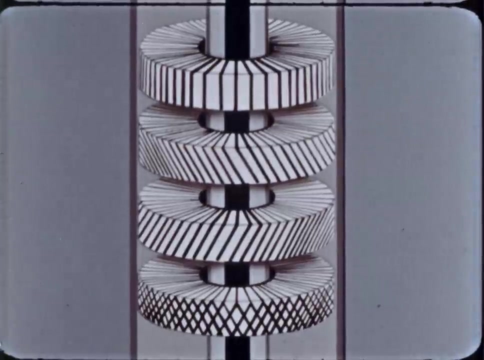 at which the reaction is slightly supercritical. Then the rods are repositioned at the critical point to hold the level of reaction constant. When the rods are reinserted fully, the reactor becomes subcritical, shutting it down. The rod movement is controlled by magnetic jacks. When coils in these jacks are 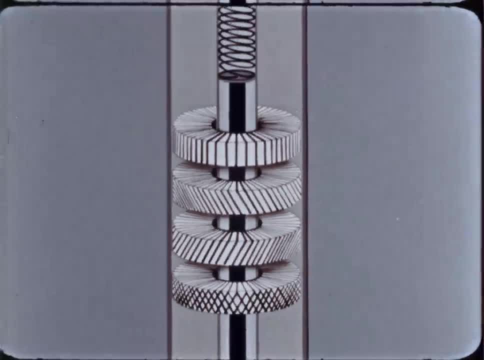 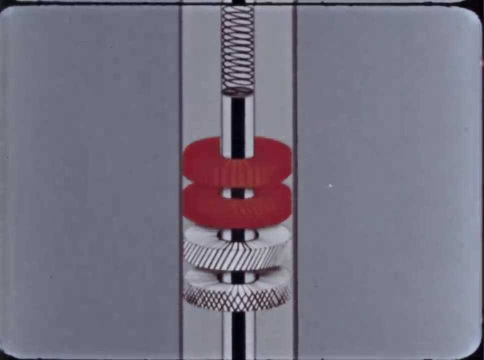 energized, they hold or move the rods. When energized, sequentially, they move the rods by increments. Gravity increases� and springs in the top of the rod housing will drop the rods if the current is cut. Loss of current scrams the reactor- a failsafe feature, Moreover. 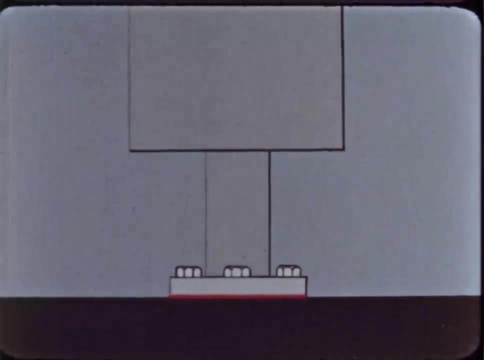 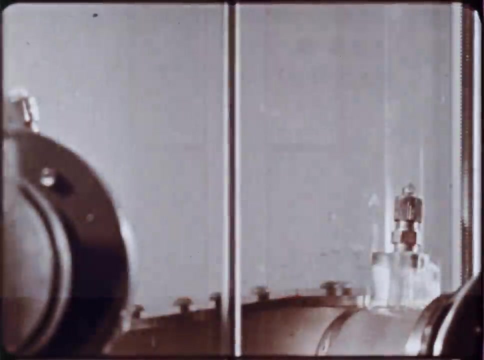 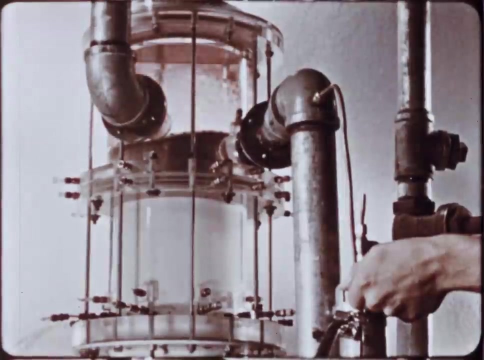 these jacks require only static seals, mainly on the pressure vessel head. No part moves against the seal, so the likelihood of leakage is minimized. As we've seen, pressurized water in the core acts as a moderator of neutrons for the 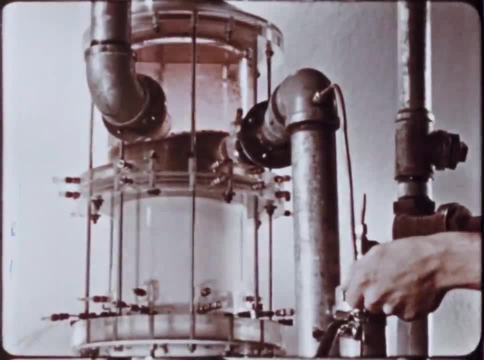 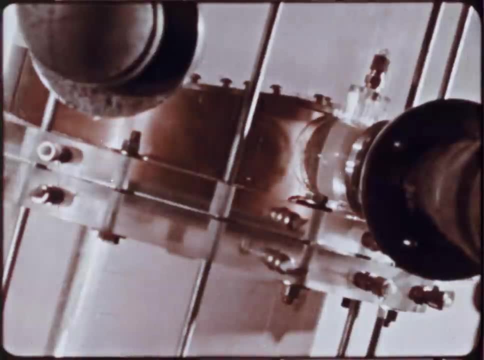 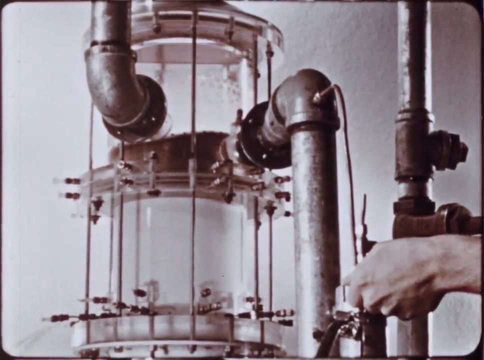 fission process, The same water transfers the heat generated in the reactor to the steam generator. With this quarter scale flow test, engineers studied the patterns of water moving through the reactor. PM1 packages have been designed so that all welding is done at the 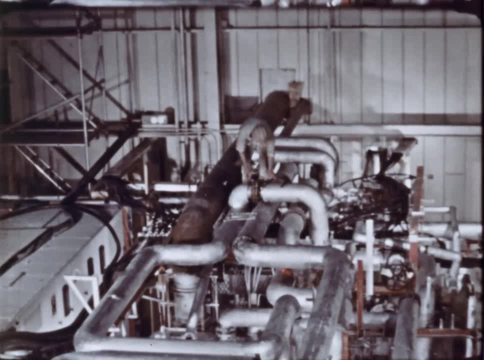 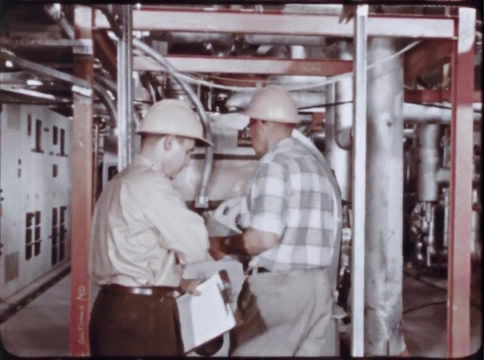 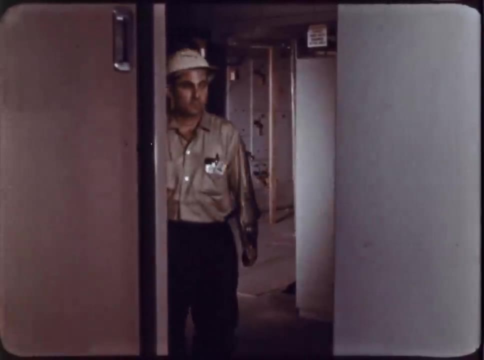 factory field welding is eliminated because flanged fittings will be used for connections to be made at the site. PM 1 was completely packaged at the contractor's plant. The packages were interconnected and tested before shipment. All 16 packages of the PM1. 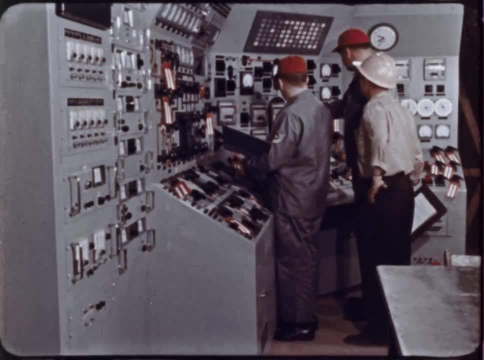 system are built to withstand the stress of airlift. The package dimensions are 8 feet 8 inches, around 45 inch wide. The system is added to the circuit in the room area and has been adjusted to match theoric city with evergreen materials. 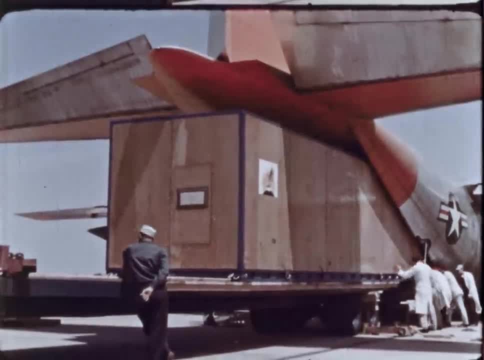 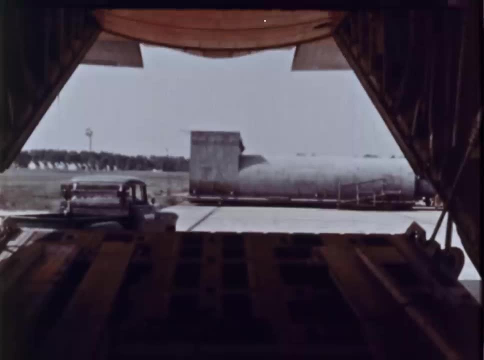 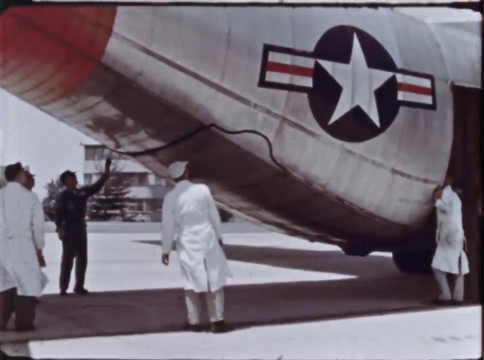 inches by 8 feet, 8 inches by 30 feet long. The maximum weight of the packages has been set at 30,000 pounds, set on the basis of the permissible load that can be carried on a C-130 aircraft on a thousand mile mission Air. 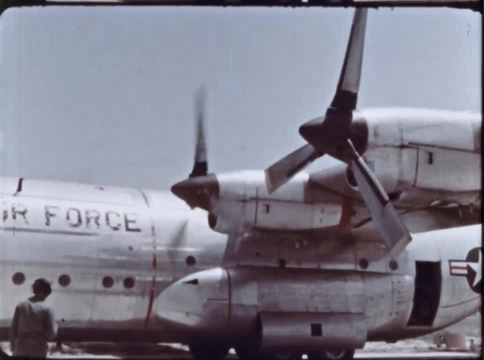 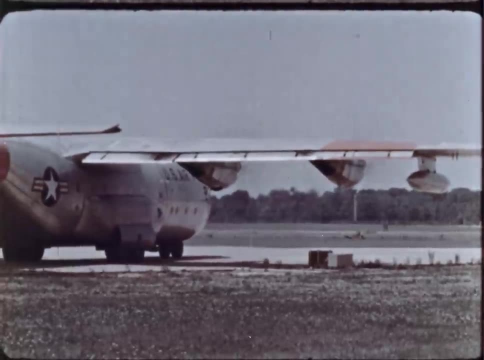 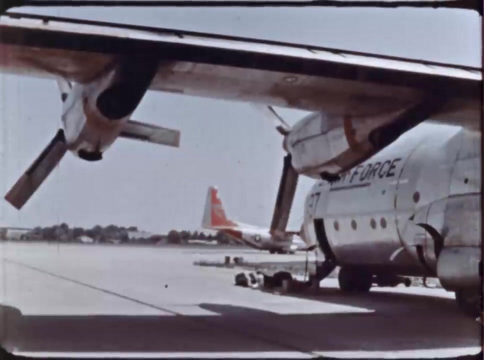 transportability of the system was flight tested during the spring of 1960. This airlift was a high point of the Air Force participation in the PM-1 project. The Air Force also contributed project officers to the program and tested the system condensers in the environmental hangars at Eglin Air Force Base. 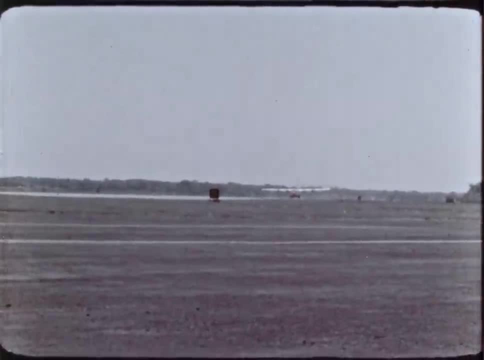 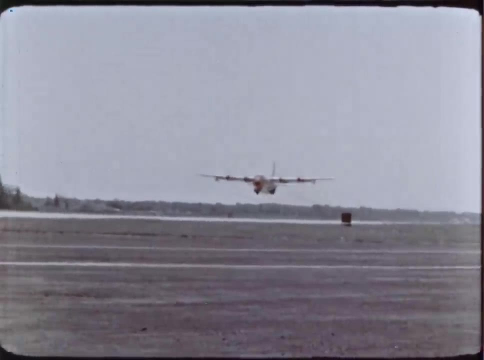 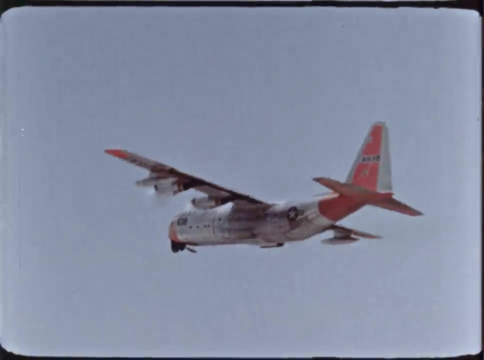 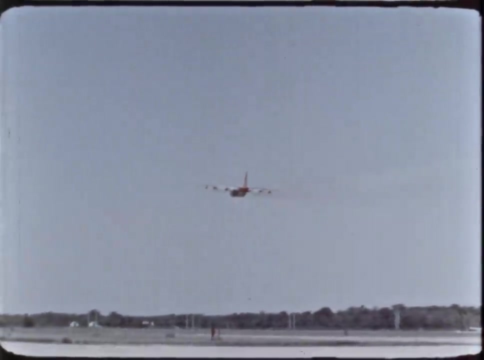 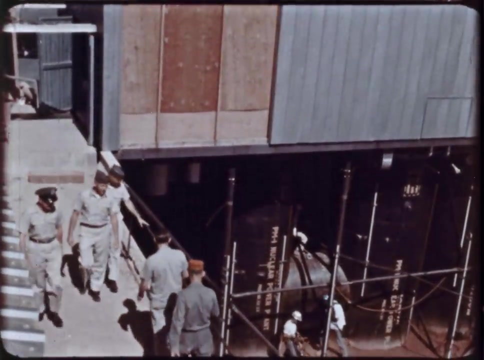 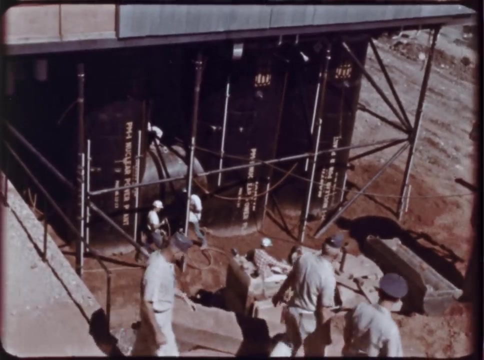 Beginning May 29th 1961, C-130 aircraft flew PM-1 packages to Ellsworth Air Force Base, South Dakota, for the overland trip to Warren Peak In 19'red, 45 minutes before take-off, C-130 aircraft landing L登 v. 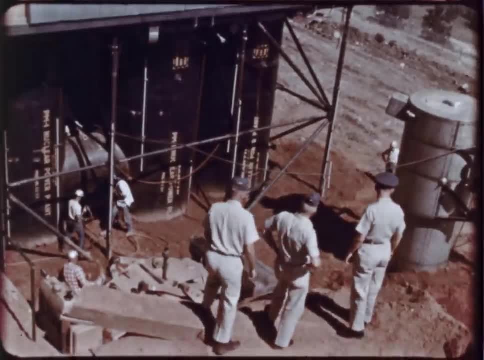 The Pam1 was reassembled at the site on previously prepared foundations. The four tanks of the primary system were erected on foundations 30 feet below floor level. Backfill of crushed rock is packed around the tangent precisares level. backfill have. crushed rock is packed around the тан. 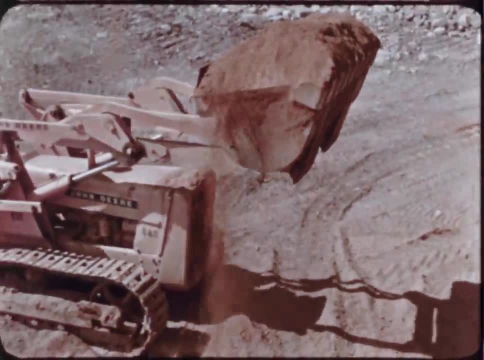 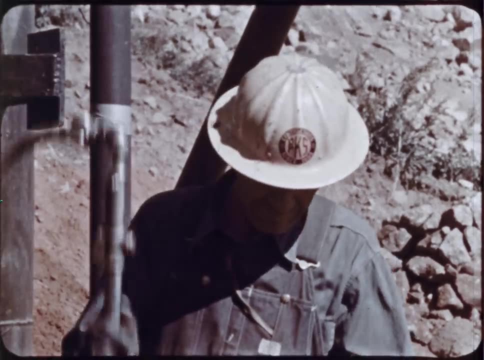 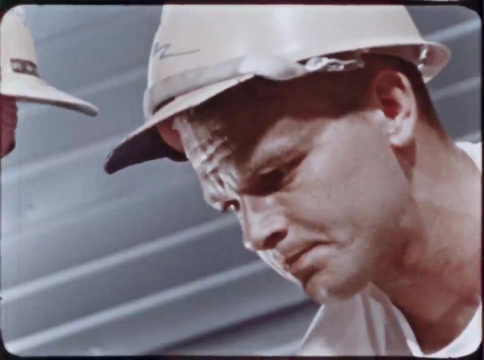 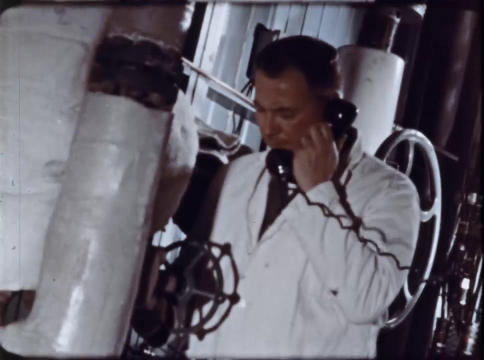 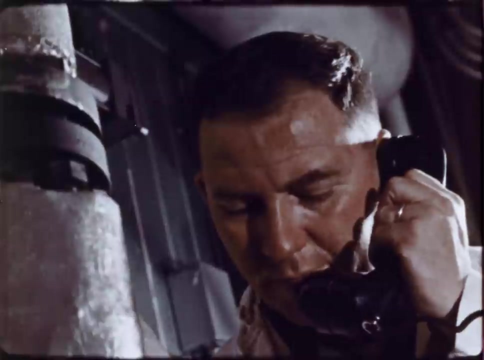 oiseep tans as a shield to reduce radiation to a safe level. Once package interconnections were complete and the core had been installed, pre-startup checkout and testing was accomplished, Subsystems were aligned in preparation for PM1 to take over its role as power plant for the site. 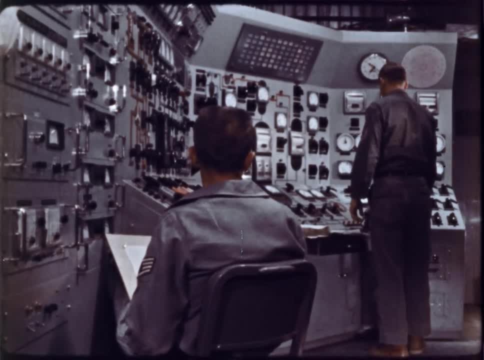 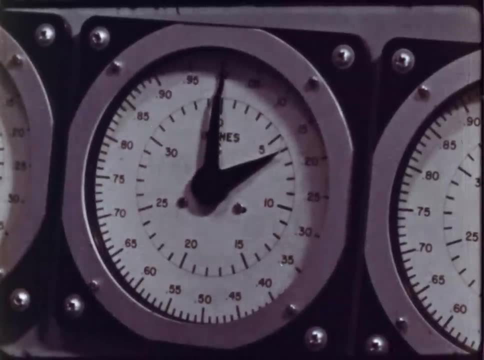 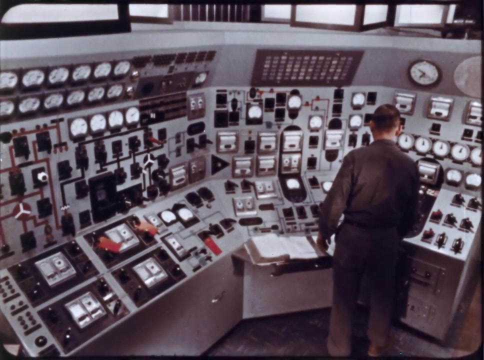 The auxiliary systems have been started and we're ready to go critical. The rods are withdrawn in pre-calculated amounts and we watch for the start of a chain reaction. The reactor period is oscillating from positive to negative each time the rods are withdrawn. 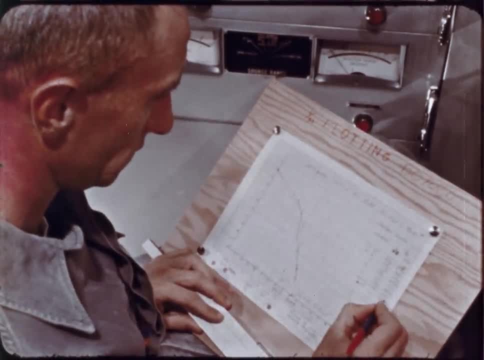 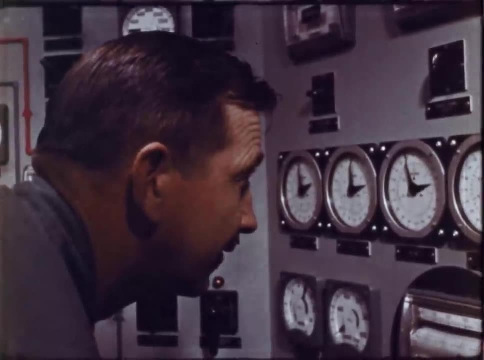 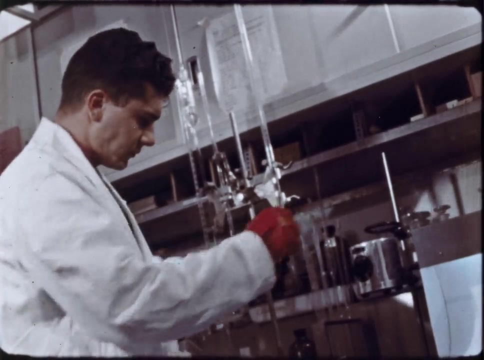 Now it remains slightly positive. We are critical. We adjust the control rods to establish the proper heating rate. The coolant water is continuously sampled so that its chemical balance can be corrected. We are up to operating pressure and temperature, ready to generate steam. 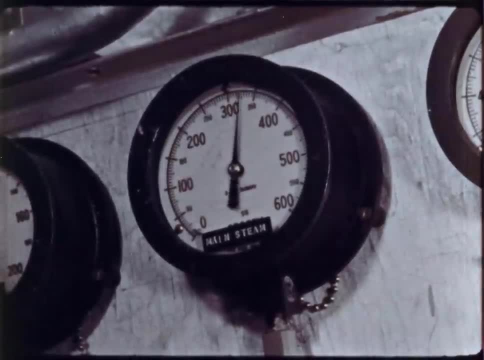 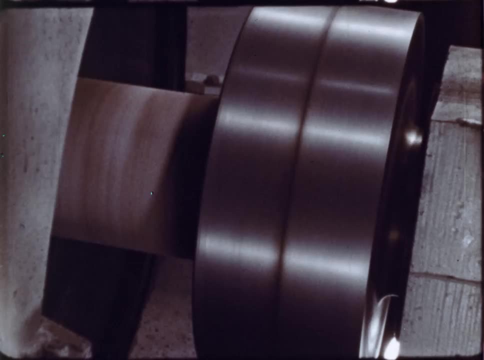 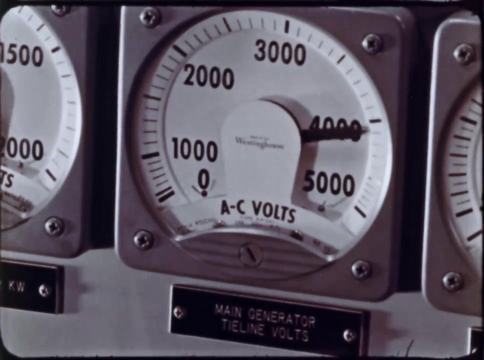 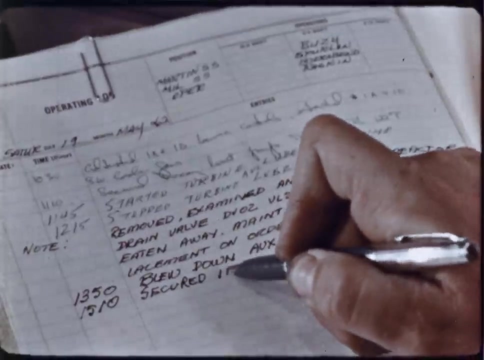 Steam to the turbine. We have the turbine up to speed Every time. the Studioscom Now apply field voltage to the generator and adjust it. Power on the tie line PM1 is in operation. Two men can operate this plant. One man monitors the plants' operation at the console. 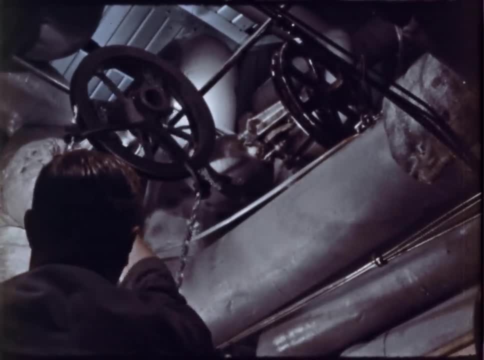 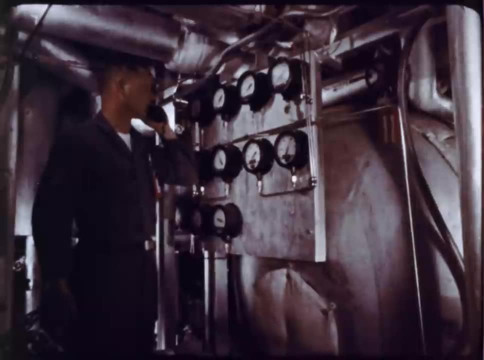 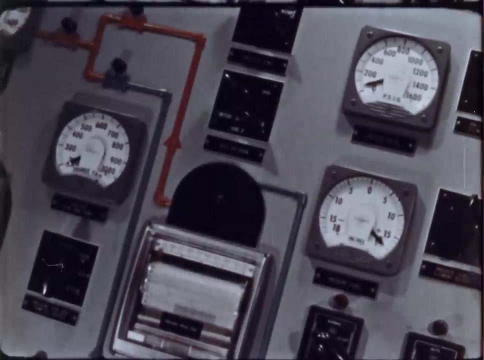 And the other continually inspects the working parts. The entire PM1 crew has been trained for every conceivable situation arising in normal operation, in emergencies or in maintenance. PM1 is a safe system. Safety is built into the fundamentals of the design. PM1 is a pressurized water system. If the water 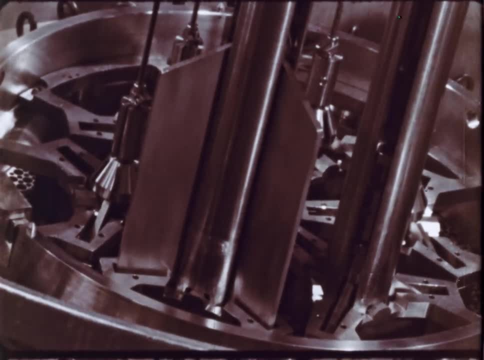 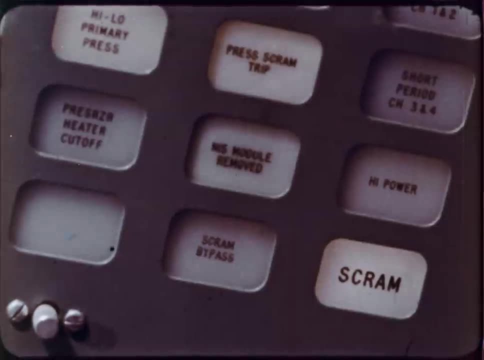 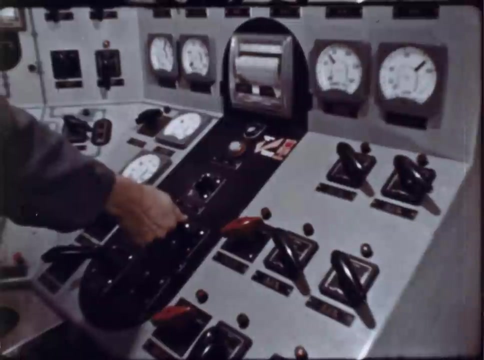 moderator in the reactor is overheated, it must expand and when its density decreases, it loses its ability to support the chain reaction. The reactor will shut down. The reactor's controls are fail-safe. If current is lost, the rods will scram the reactor. 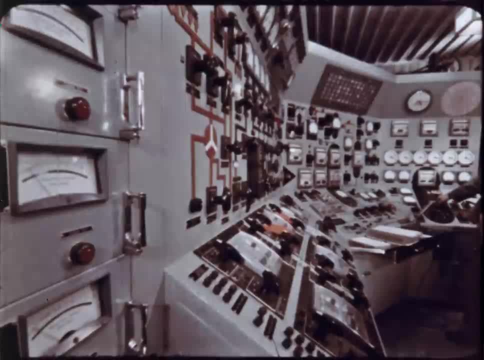 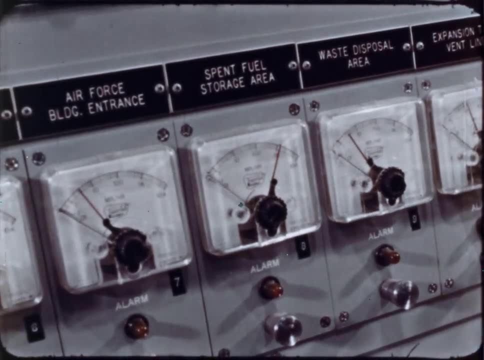 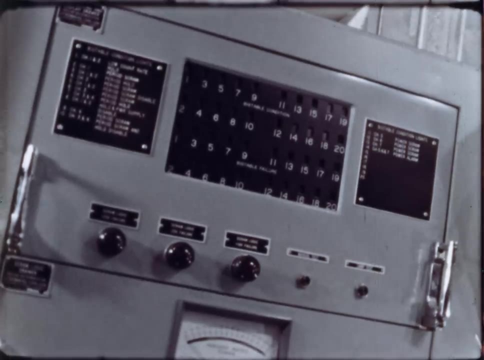 The instrumentation continuously monitors 68 points in the system: temperatures, pressures and radiation. Solid-state components ensure a high order of reliability in this instrumentation. The reactor safety system, which can warn the operator of potential trouble, also ensures that the reactor is safe from damage or damage. 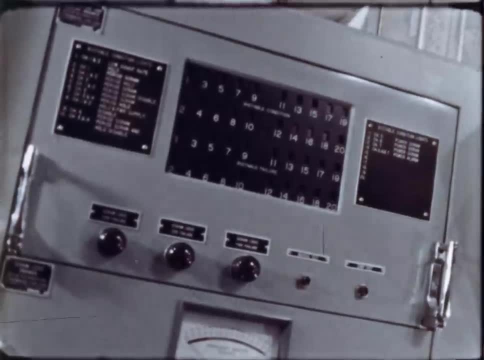 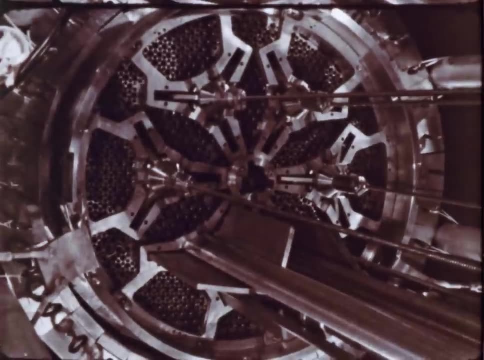 The reactor's safety system, which can warn the operator of potential trouble, incorporates the scram logic circuit. This is a self-monitoring device that watches for 13 specific combinations of conditions. Its function is instantaneous action. For example, in five sets of conditions it may lock the rods so that 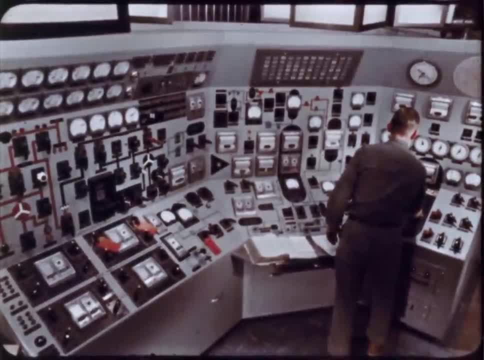 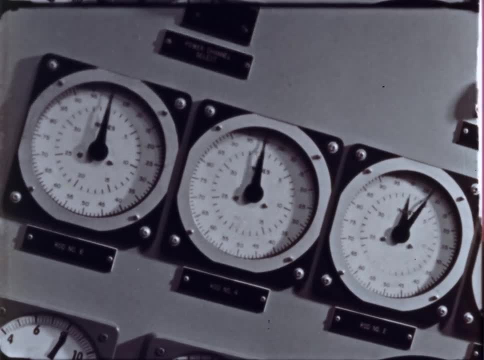 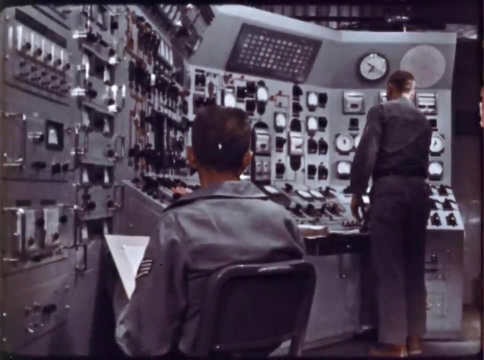 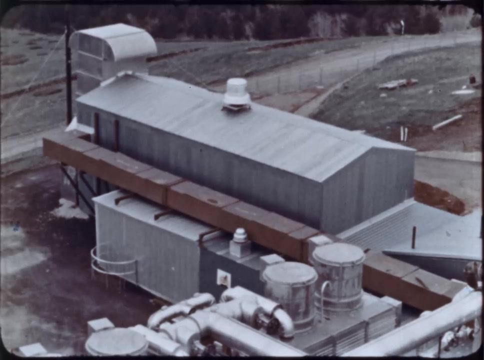 they cannot be withdrawn further, or if the reactor exceeds 125% power, the circuit will scram the reactor. The crew has been thoroughly drilled in safety until emergency procedures and corrective action are automatic. A single PM-1 core will furnish full power to the radar site for two years. During this. 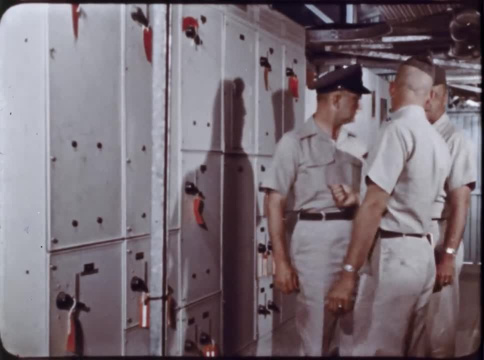 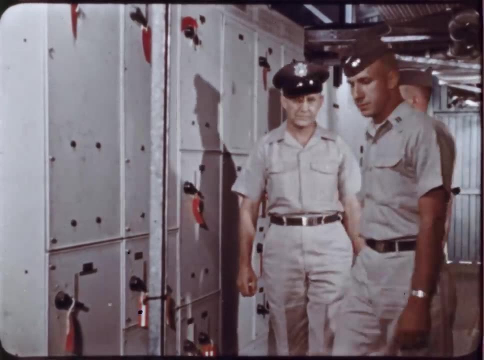 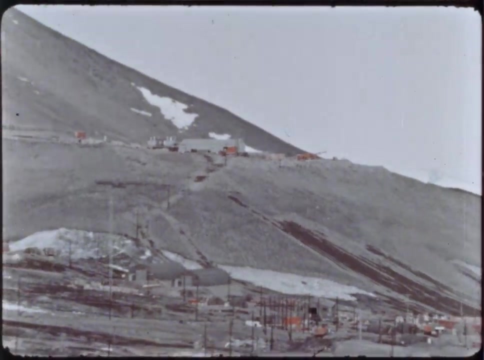 time, the Air Force, the Atomic Energy Commission and Martin will scrutinize PM-1 operation. We will discover ways to accelerate the operation of PM-1.. The first of a series of closely related systems, PM-3A, is being tested in the. 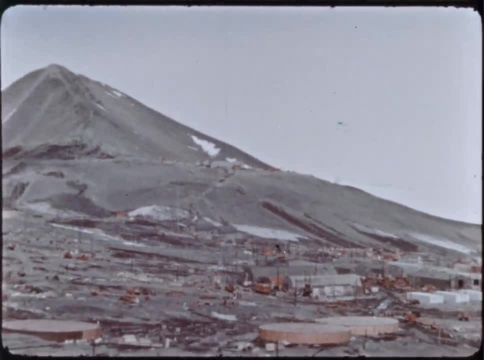 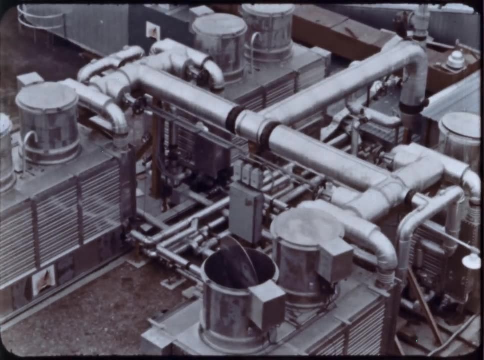 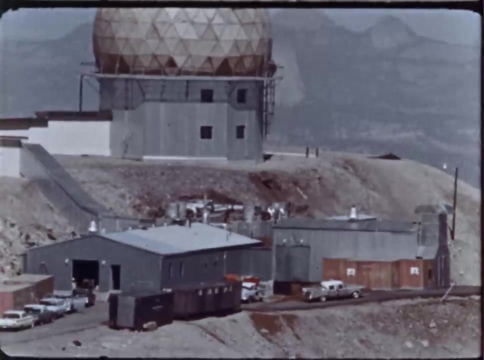 Antarctic. Compact and self-sufficient portable plants installed in remote regions difficult to supply are pioneers. PM-1 and its small crew is proving the safety and practicality of the medium-range reactor power plant. PM-1 opens the frontier for many new applications of nuclear electric power, both military and civilian Music Music.